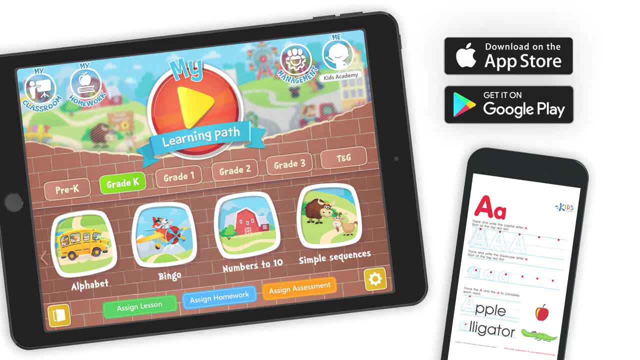 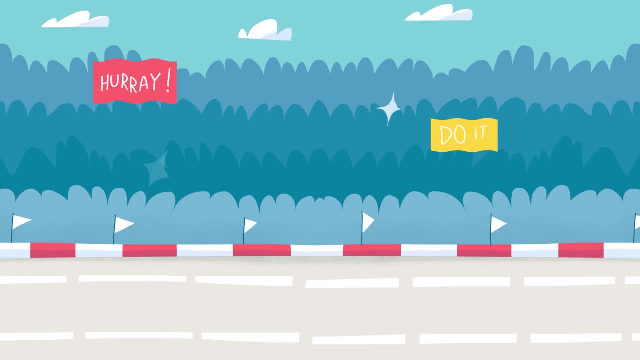 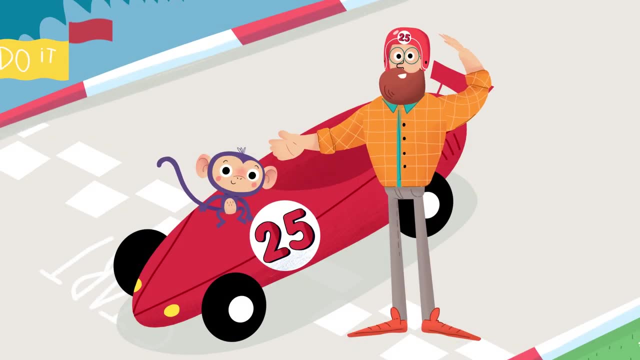 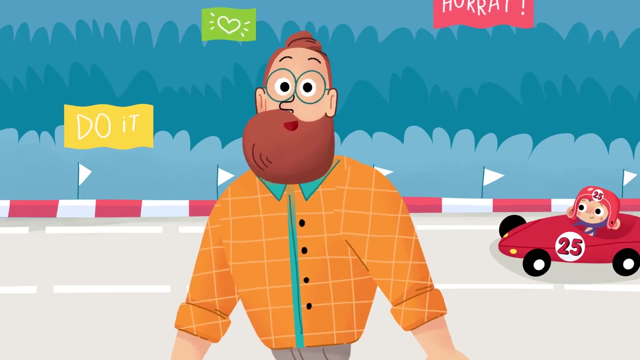 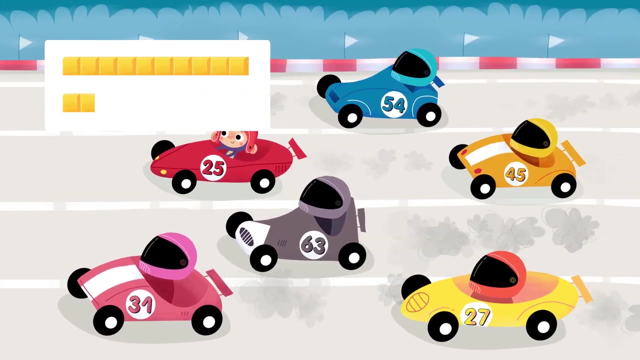 Hello boys and girls. We are at the racetrack ready to compare some numbers. Let's see which cars participate in the race today and which numbers we are going to compare. You already know about place value and can compare numbers using base 10 blocks. Now I'll help you find. 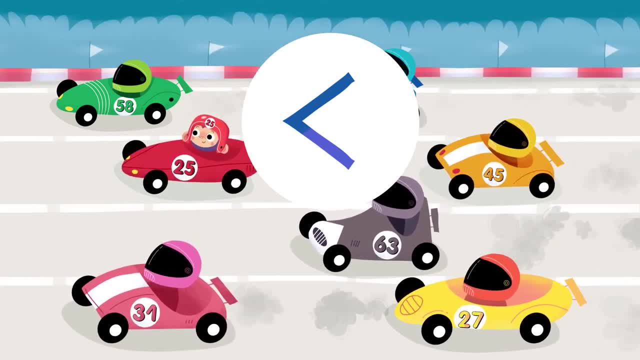 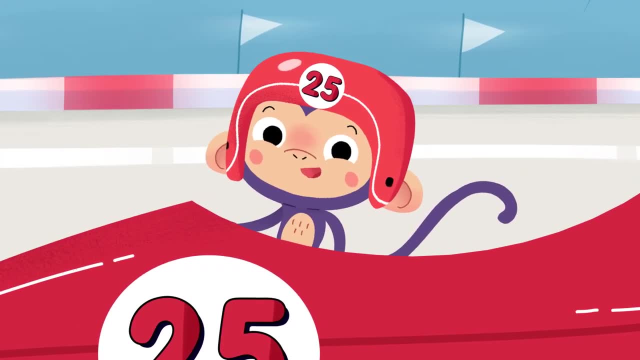 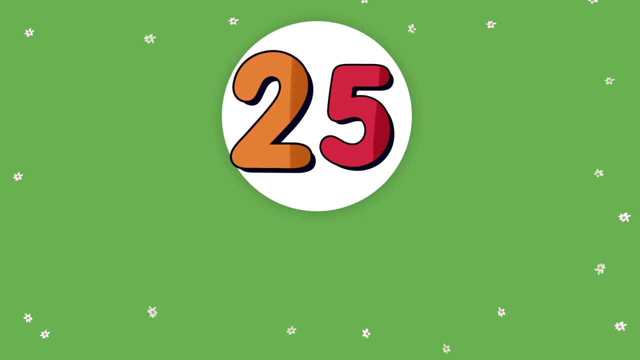 numbers that are greater than or less than other numbers On your mark. get set, go. Do you like that racing helmet? See the number. It's number 25.. We can look at the digit in the tens place first to help compare numbers. How many tens does my number have? 25 has. 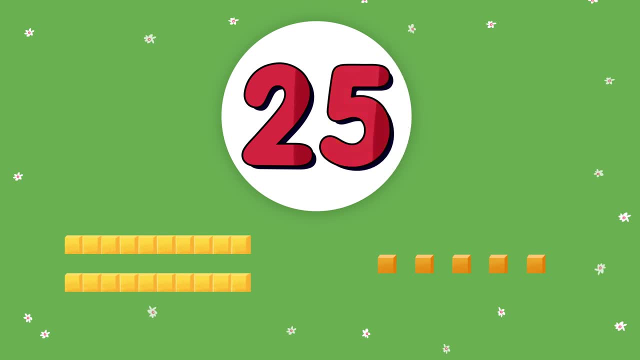 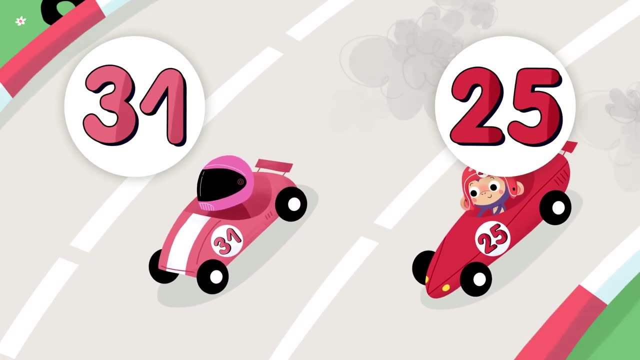 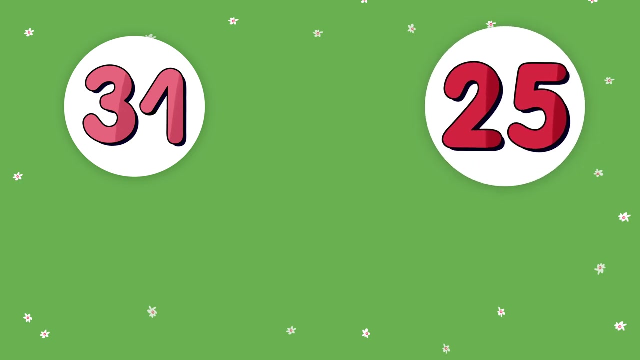 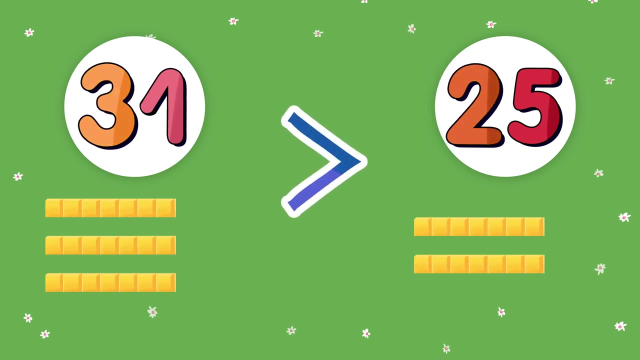 two tens, It also has five ones. Nice job. There's one of the race cars. now What number is it? Is 31 greater or less than 25? Both 25 and 31 have numbers in the tens place. See, We see that 3 is greater than 2.. That means that 31 is greater than 25.. We put up. 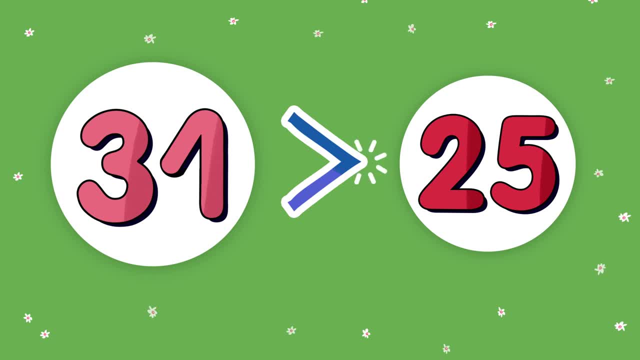 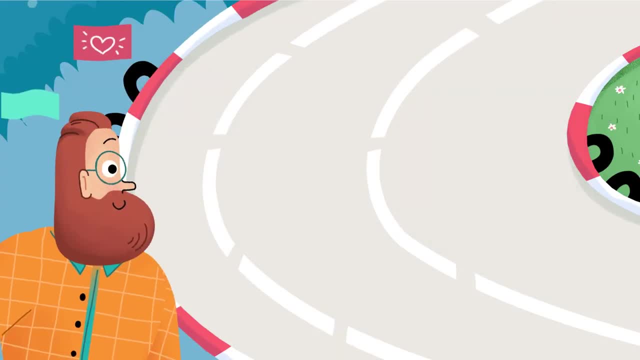 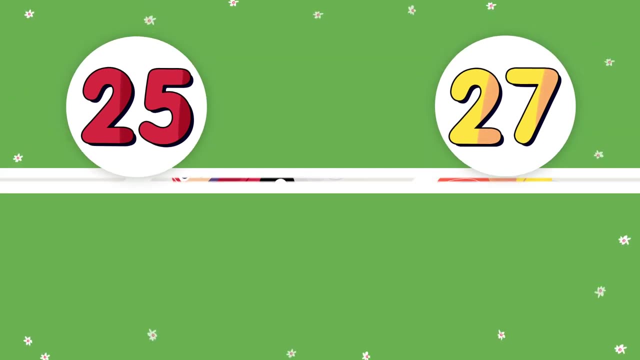 the greater than sign, with the small pointed side facing the smaller number. So the sign would look like this: Whoa, look, There's another car with a new number. Is that number greater than 25?? Well, First we can look at the largest place, which are the numbers on the far left. They're the 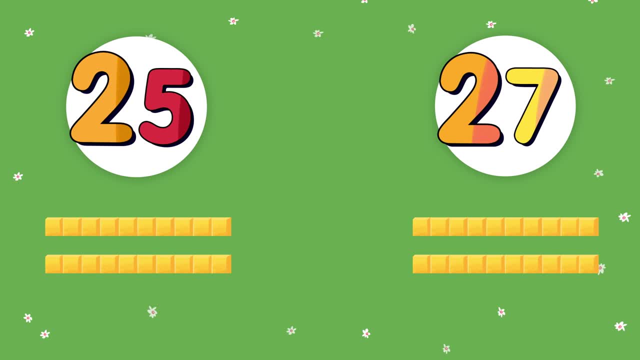 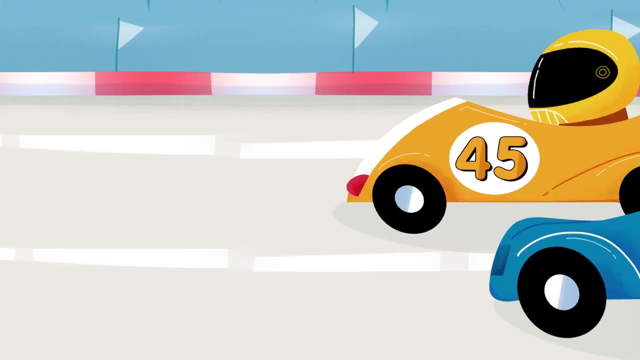 same, They're both 2.. That's okay. If the tens place is the same, then we can just compare the ones place. See, We can compare using place value. I can hear some cars getting ready to race. Let's compare their numbers. Do you remember where we start when we compare? 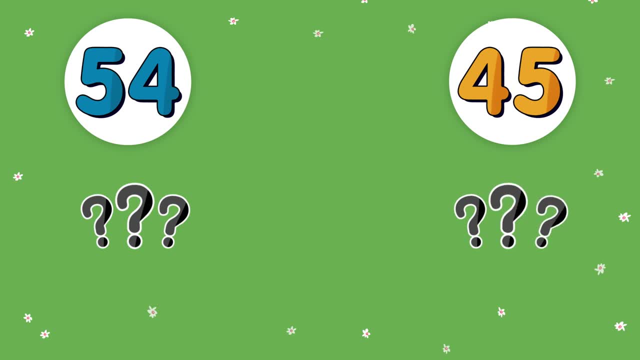